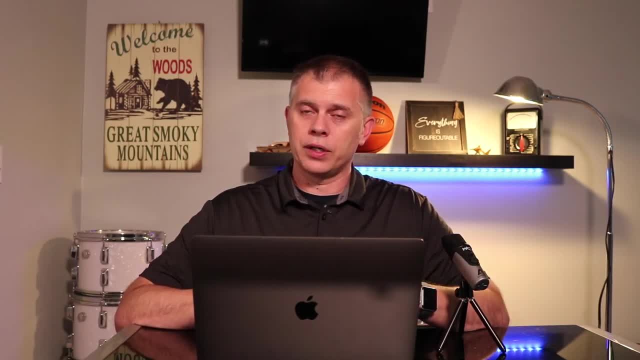 to take calculus 1,, calculus 2, calculus 3, sometimes differential equations and then some type of calculus-based science like calculus-based physics 1,, 2, and 3.. Now there are some engineering programs now that are looking to start students a little earlier, so you might take an introduction. 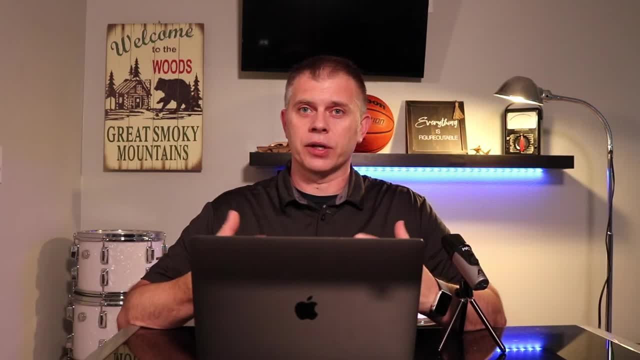 to engineering class, or maybe another type of introductory class, while you're taking these math and science classes. Now, when we look into this, you'll see that there really is not a two-year theoretical engineering degree. What there is is a two-year pre-engineering. 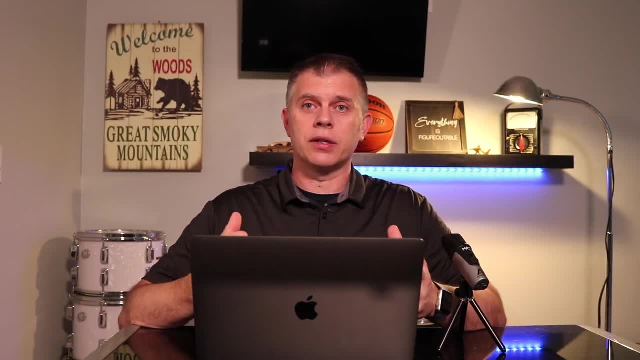 degree. The reason for this is because, generally, engineering students spend their first two years taking gen eds, taking all their math, all their science, all their math, all their sciences and all their gen eds before getting into the engineering programs years 3 and 4. It just doesn't make a lot of sense that a community college 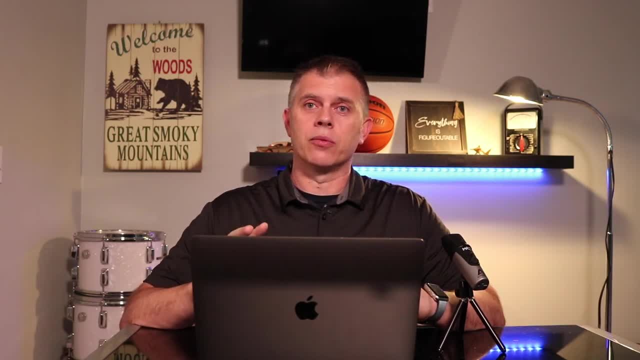 would offer a two-year theoretical engineering degree, when the first two years is spent taking math classes. So what community colleges will do in this case is offer a pre-engineering degree, and so a student can actually go to a community college. They can take all their. 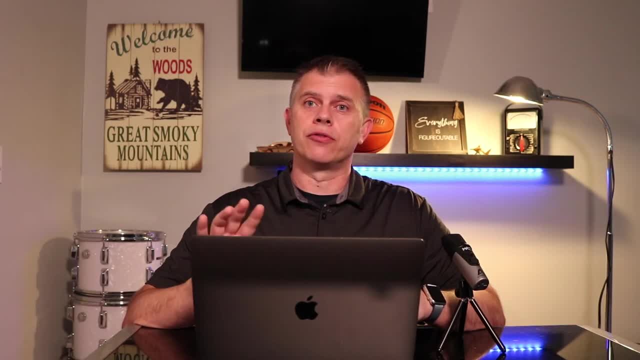 math and science classes. get those out of the way, transfer to a four-year university and then all they have to take are core classes, their core classes at the university. So now let's look at a four-year engineering technology degree. Now remember what I told you: that somebody who graduates with an engineering technology 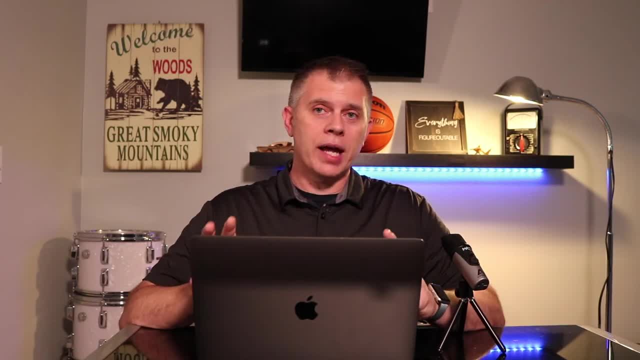 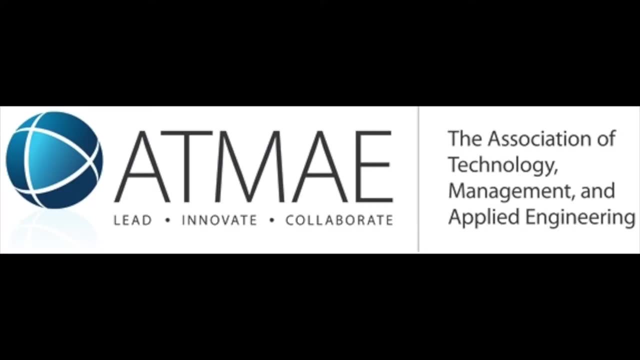 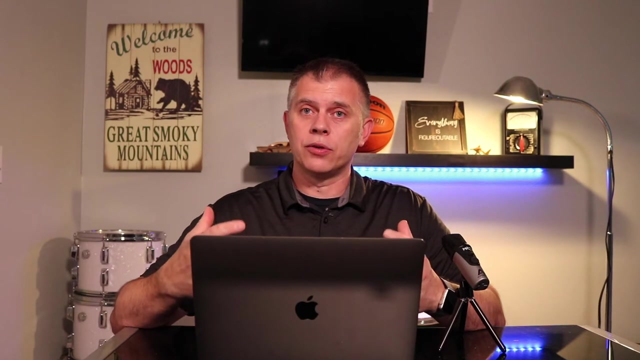 degree, according to ABET, is a technologist. A better name for engineering technology is applied engineering. As a matter of fact, there's another accrediting agency named ATME, which stands for the Association of Technology Management and Applied Engineering, who did a lot of work to come up with this new division of applied engineering. instead of just 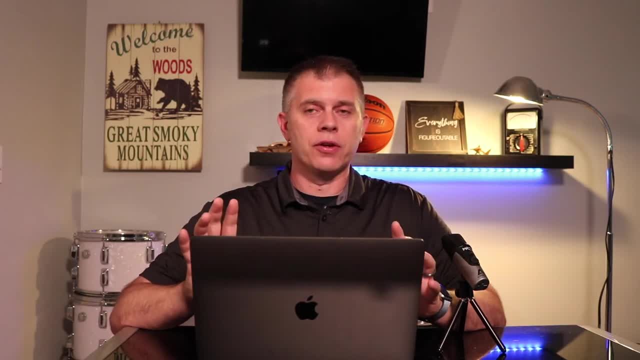 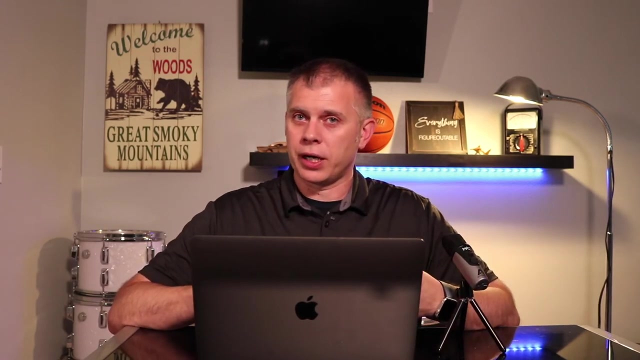 engineering technology. Now, one thing to understand is there's still theory in engineering technology, but there is not as much math and science in engineering technology as there is in a theoretical engineering program. So generally, students who take an engineering technology program will take college: algebra, trigonometry, statics, calculus, sometimes calculus. 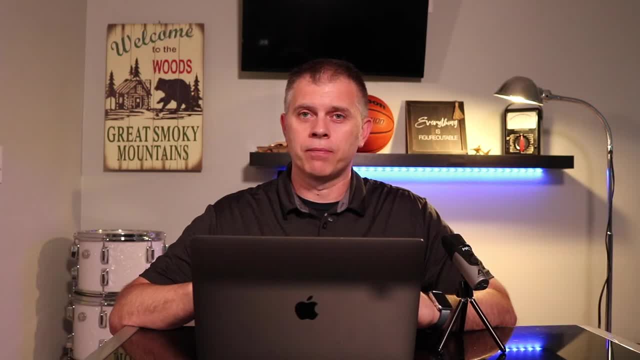 2. that's generally the most math you'll have to take is calculus 2.. Then they'll they'll have to take some type of sciences, but generally those sciences are algebra based. Now that is not saying that a student can't take a calculus based science class. That's perfectly. 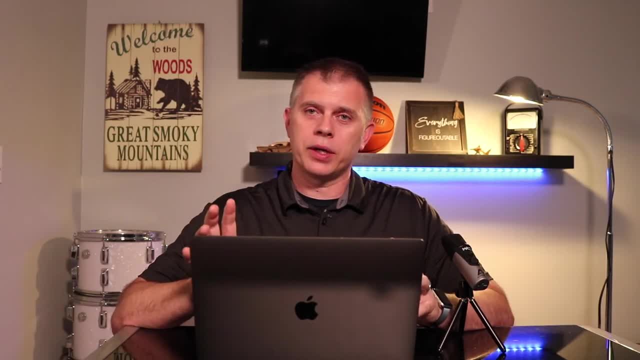 fine for a student to do that. But one of the biggest differences between an engineering technology program and a theoretical engineering program is the hands-on, the applications. That is why engineering technology is considered applied engineering, whereas regular engineering- I'll call it- is considered theoretical engineering. So you can expect labs in an 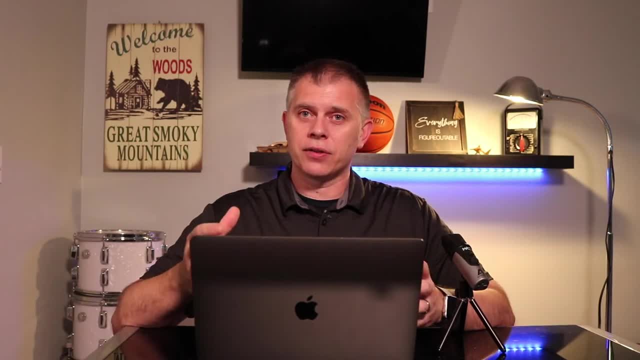 engineering technology program to have a lot of applications based on the industry that they're going into My students, for instance, we focus a lot on automation, So generally the labs in my classes are heavily focused on POCs, robotics, mechatronics, any type of automation that they'll. 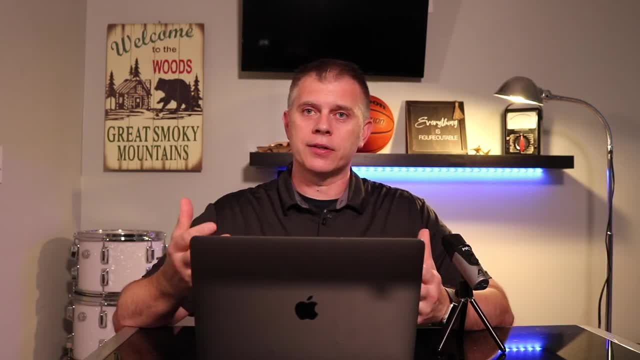 find in industry, So that way they are better prepared when they go into industry to have this real-world applications. Now let's look at a two-year engineering technology degree. Remember I told you a two-year engineering degree. Well, someone can actually receive a two-year engineering technology degree in. 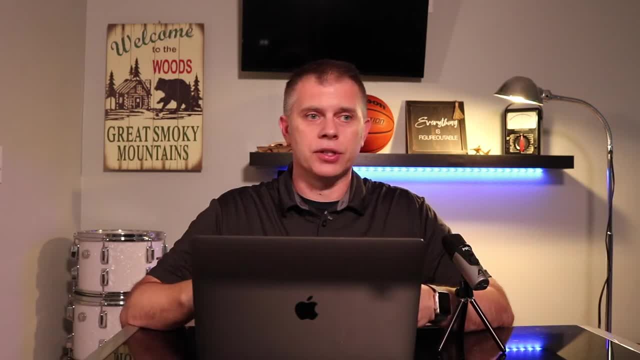 electrical engineering or automation engineering or mechanical engineering technology from a community college. So generally they will have an associate of applied science or an associate of science degree in electrical engineering technology or mechanical engineering technology and so on. I actually have an associate in engineering technology and that is really. 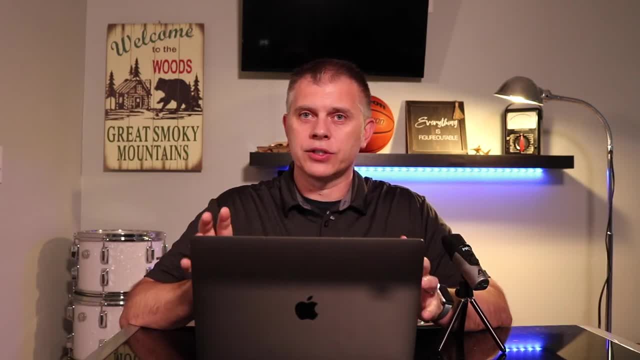 what causes so much confusion when you look at a four-year engineering technology degree. Many times I will have students come to me and they will think that they're getting a four-year degree but they're going to be a technician in the field. Well, that's possible, They could be a technician. 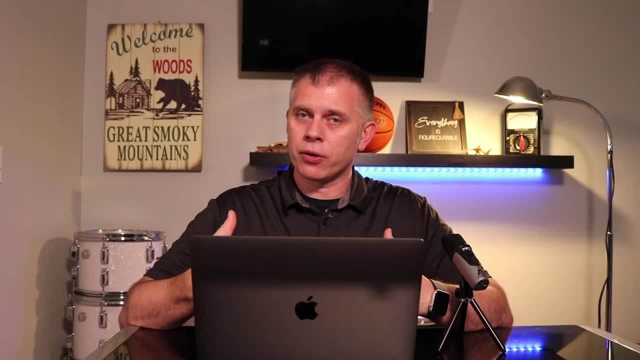 but what I've seen is the majority of the students that graduate with my program with a four-year engineering technology degree receive positions as engineers. Now, like I mentioned before, both the two-year engineering technology degree, a four-year engineering technology degree and a theoretical engineering degree can be accredited through ABET, but only the two-year. 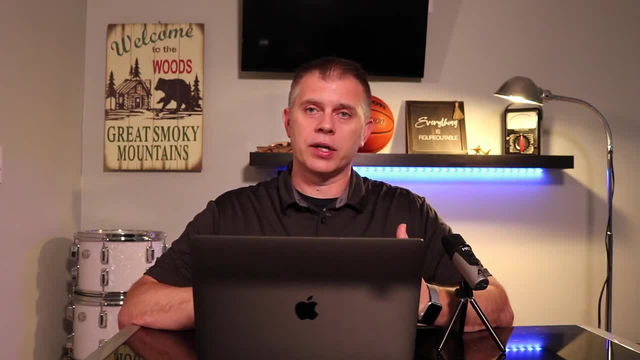 engineering technology and four-year engineering technology can be accredited through APMEI. So there are plus and minuses to both. So let me just break this down real quick and help you understand the differences. Now, if you go to a community college and you get a two-year, 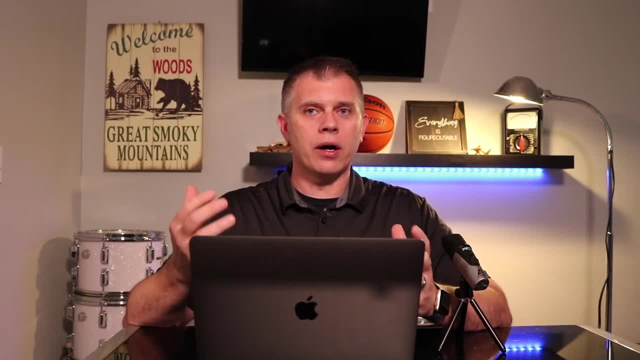 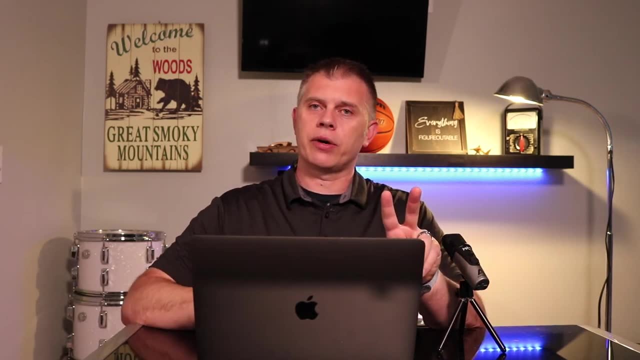 engineering technology degree. a lot of times you can have what we call articulation agreements or a two plus two. What that means is you take two years at the community college and then transfer into a university and get the other two years at the university and end up with 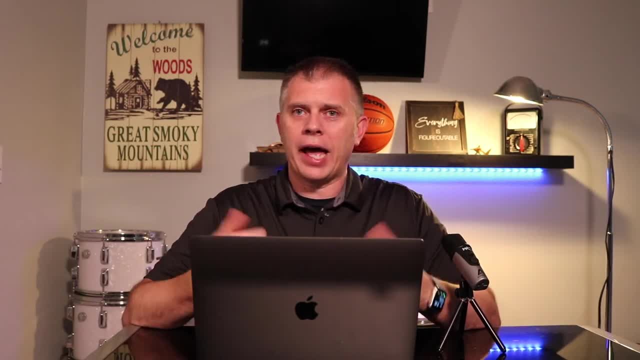 your bachelor of science degree in engineering technology. A graduate actually receives an associate of applied science and an engineering technology degree and a bachelor of science and engineering technology degree. Now is that really beneficial? Maybe It could be, So. one way that this could be beneficial is you go to a community college where sometimes 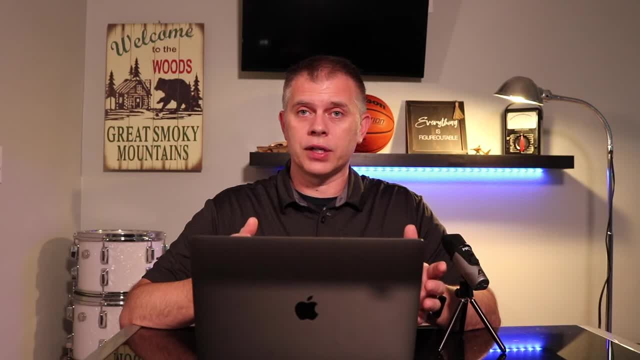 it's free and many times it's way cheaper than a university- and then receive your associate degree, Transfer to a university, actually have a job as a technician while you're finishing your bachelor degree. Sometimes that company might even pay for your degree One way or 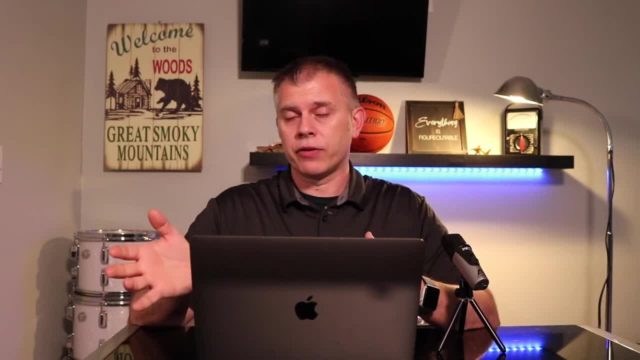 the other, you're making quite a bit of money as a technician while you're finishing up your bachelor degree. Now, that's not always feasible because, honestly, being a technician takes a lot of time, but you will make quite a bit of money. Now, if you're looking at 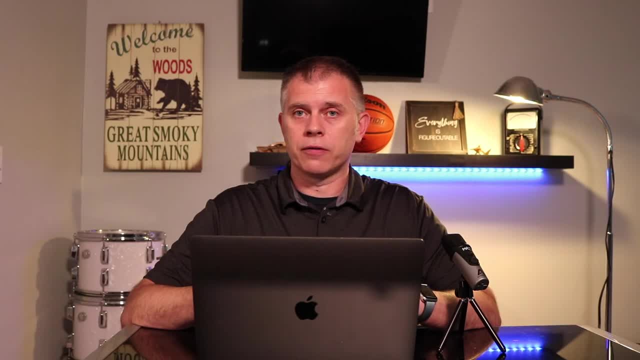 being a technician, then really all you'll need to do is get a two-year degree from associate degree. If you want to be an engineer, then you will need a four-year degree. There's no doubt about that, One of the downfalls of a four-year engineering technology degree. 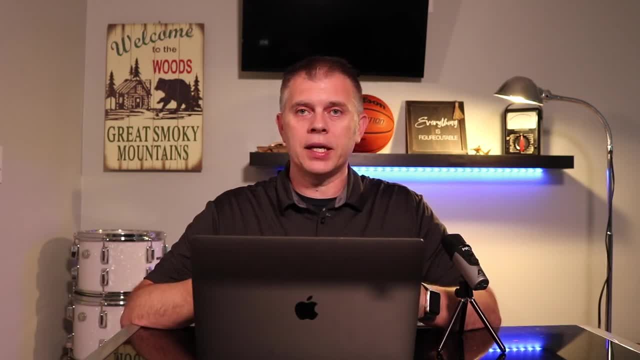 is the ability to get your PE licensure. PE is professional engineer and a lot of times jobs require a PE licensure. Now it depends on the state for PE licensure, but some states don't accept that. I'll teach in a state that does not accept an engineering technology. 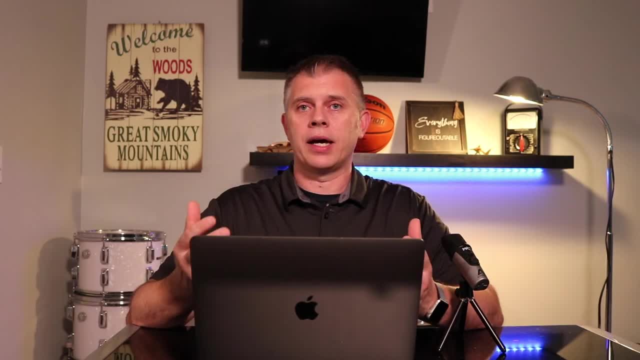 degree in order to be able to sit for your PE licensure Now, generally that doesn't matter so much. Students in my program are getting high paying jobs and they don't have any trouble at all getting the job, So that has not been a factor. 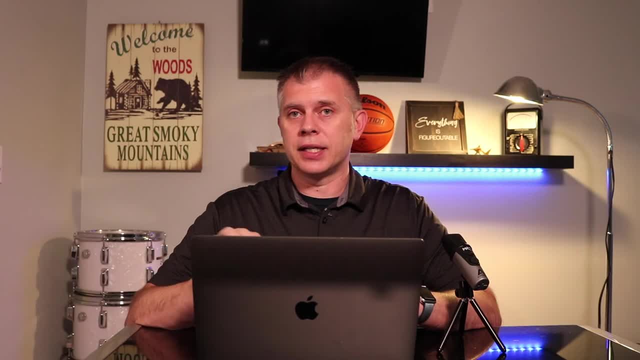 at all. in the case of my graduates Now, I will say I teach in a niche program. As I mentioned, it's more of an automation engineering technology program. The demand is very high, and so that might be the big difference, for instance, why my students don't need a PE licensure. 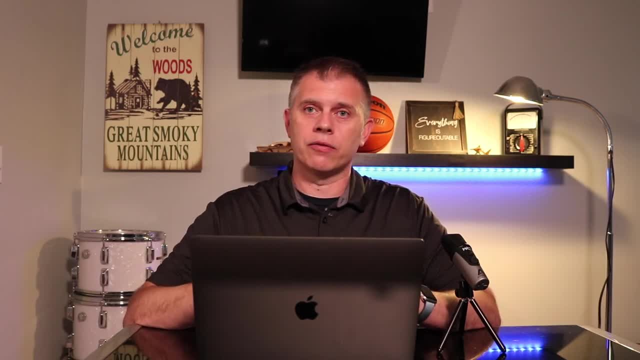 as much, But that is a downfall. You need to do your research on that. So if you're in a state that accepts an ABET accredited engineering technology degree for PE licensure, then you really don't have anything to worry about. The only difference between that is: 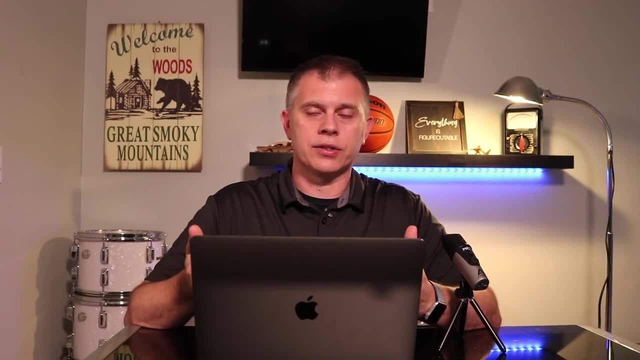 you will have to work a little more in industry before you can sit for that licensure. But there are some states- and again you need to check in on this- there are some states that do not allow a graduate of an engineering technology degree to sit for the PE licensure. 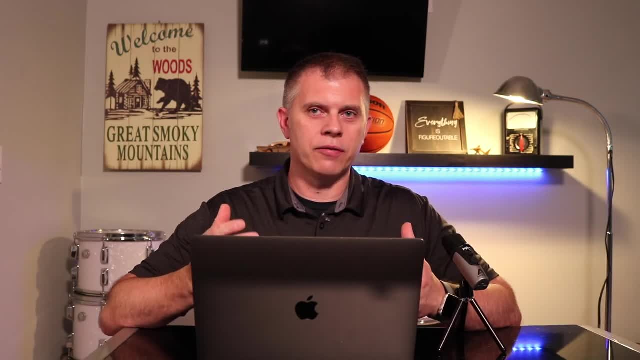 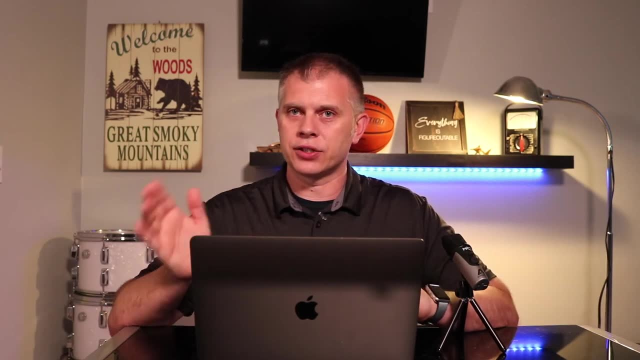 So let's look at these titles that ABET placed on these graduates of engineering, technology and engineering degrees. Again, remember, a two-year engineering technology degree will lead to a technician position. According to ABET, a four-year engineering technology degree leads to a technologist. 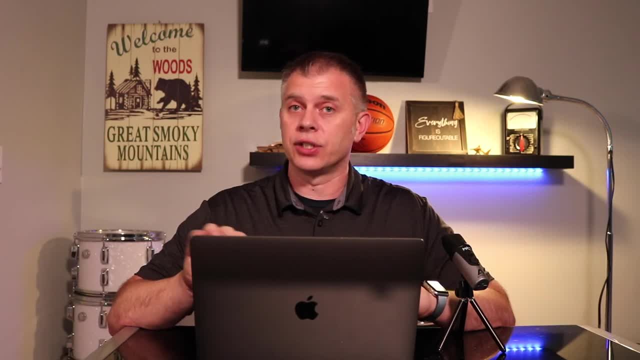 While a four-year theoretical degree leads to an engineer. Now here's the issue with that. I challenge you: go to monstercom or indeedcom or one of these websites where you can look up positions and type in the term technologist and tell me how many engineering. 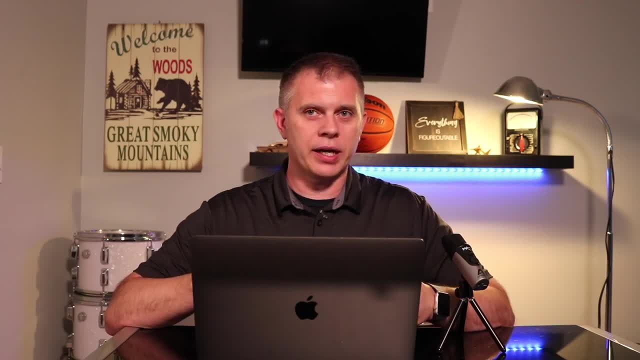 positions come up. Generally, what you're going to find is very specialized positions or medical positions. You're not going to see technologist positions out there for engineers- Again, what I've seen- the majority of my students- they receive jobs as automation. 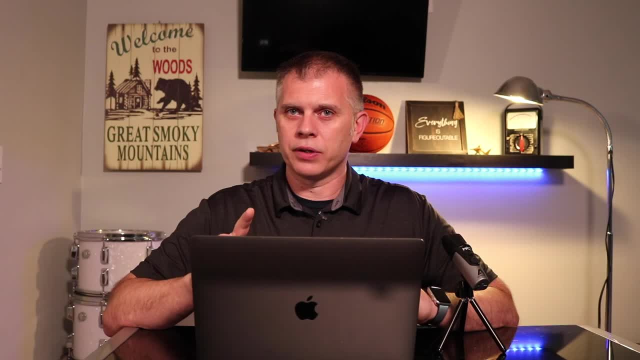 engineers. They're not technologists. which leads me to the last point in this video. If you get a two-year degree and you go out into the field and you're a technician and you love your job, you're going to have a very high paying, very good job There is. 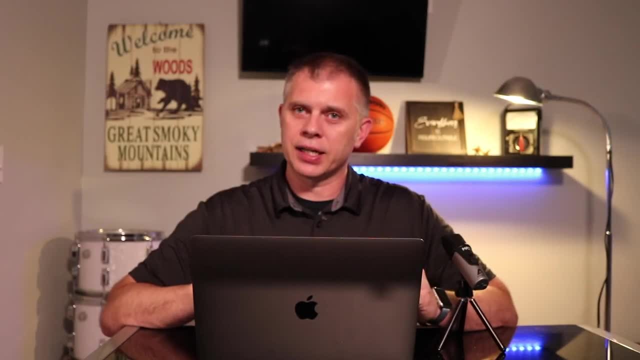 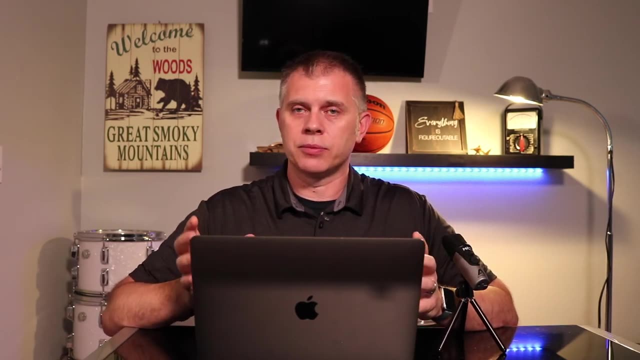 absolutely nothing wrong with that. If you get a four-year engineering technology degree and go out and get a job as an engineer and you love your job, then that's fantastic. Here's what I've seen my students get jobs in as far as salary goes On the low end. I've seen $55,000 up to $85,000 starting out. That is in the lower end. So if you're in the lower end, you're going to have a very high paying job. You're going to have a very 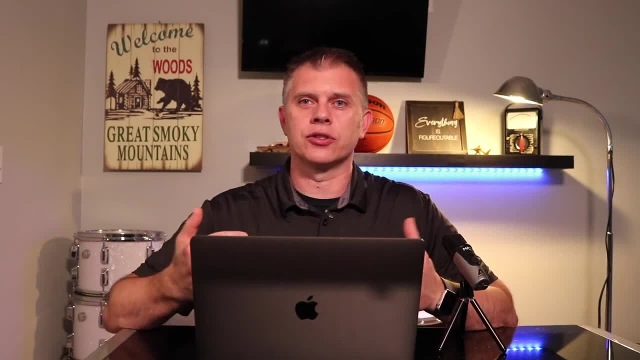 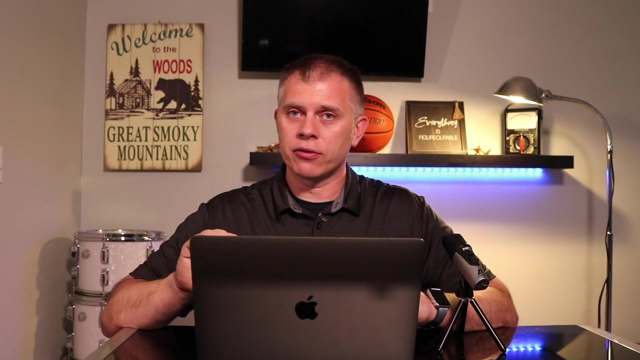 good job. That's in automation engineering. Sometimes this is called something different, like controls engineering or instrumentation and controls, which is my background, But these are very high paying jobs. So the question that you need to ask yourself is that which one is the best fit for you? Are you a better fit as a technician, If you don't mind getting? 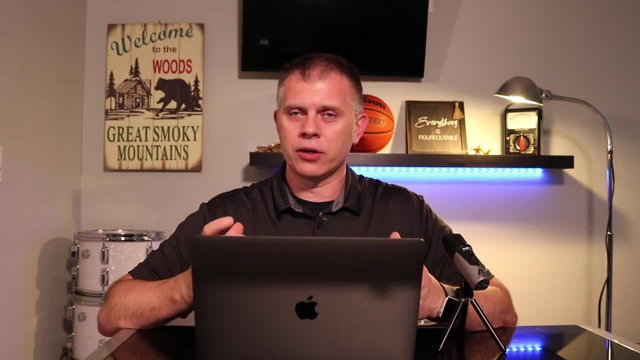 dirty and you really like getting your hands on things and fixing things, then you might be a great technician. If you like the design of things but maybe you want more of an office type job, An engineer might be a better fit for you. Both are fine. I have honestly seen cases. 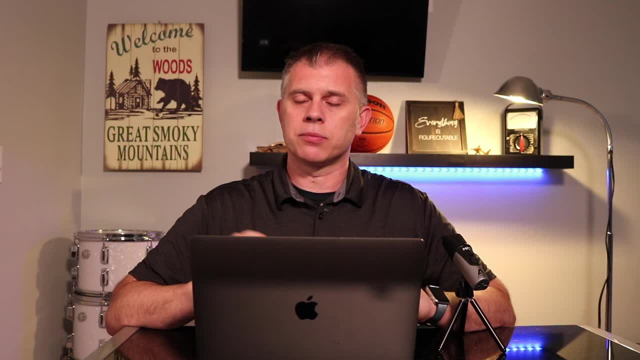 in industry where a technician will make more than an engineer, because many times technicians are paid by the hour while engineers are paid by salary, And of course that opens up the doors for bonuses and different things. But a lot of times you'll have a technician and